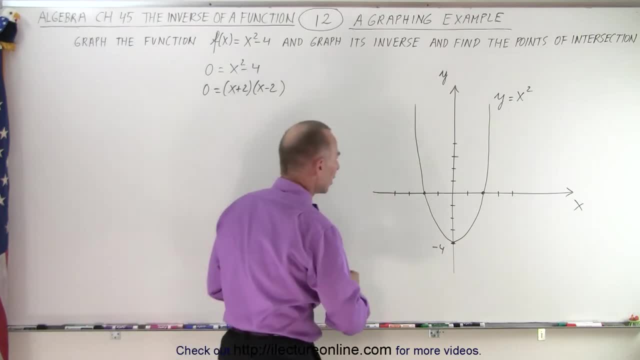 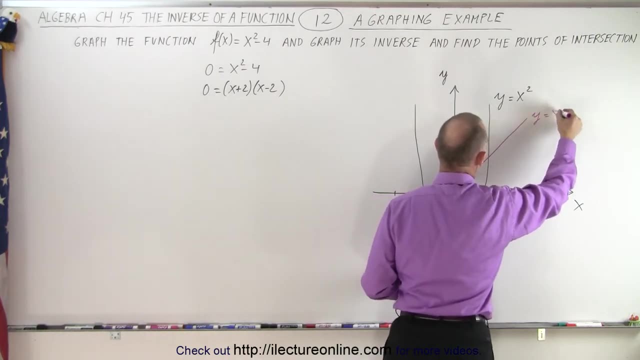 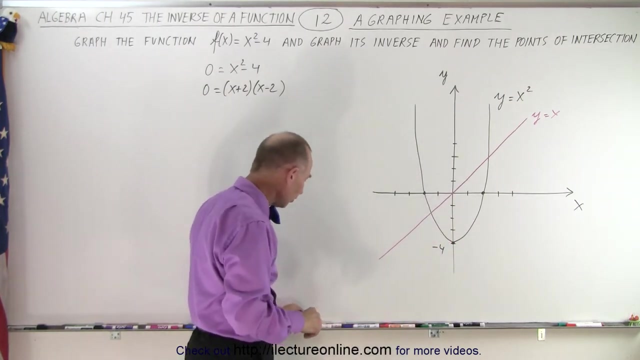 the inverse. well, first of all, we can, we can draw the y equals x x line, that's the 45 degree line, like this: so this is the y equals x line, and come back on the other side, right here, like that, all right, and notice that if- and let me look for my green pen, notice that if the vertex is at minus, 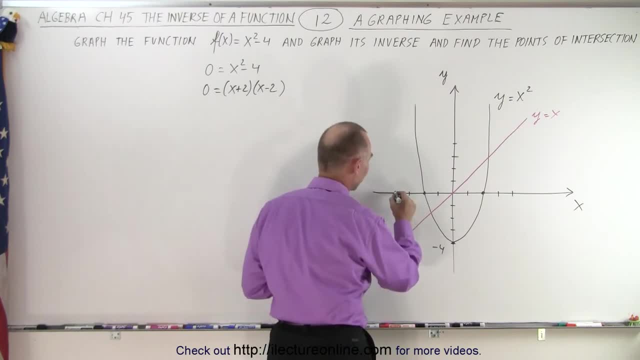 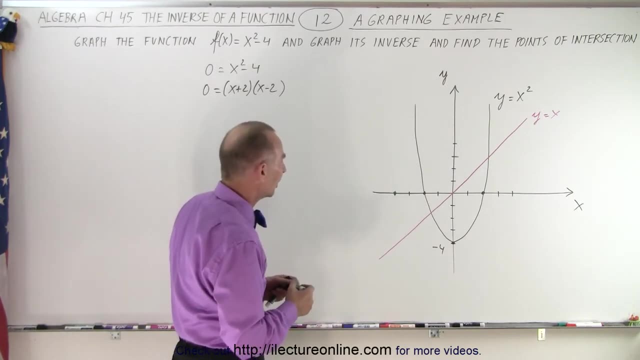 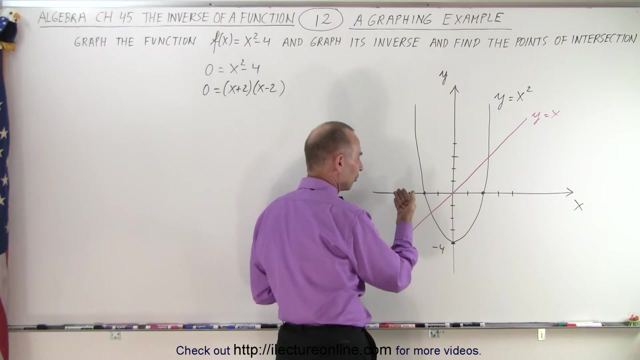 four on the x-axis, it will be at minus four on the y-axis. that means that the vertex of the of the graph that is represented by the inverse of the function is going to start at this point, right there. now we know that this inverse of the function will cross the y equals x line at the. 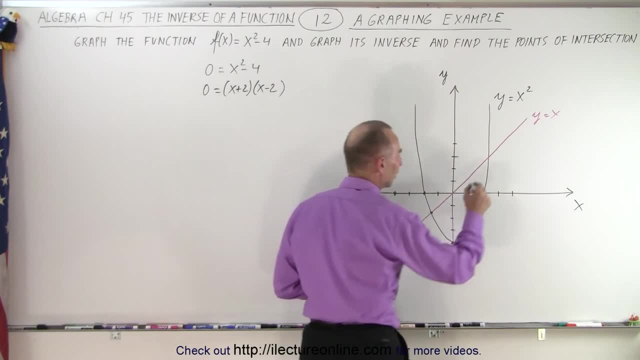 very same point as the function itself and it should cross there as well. so that means that if i now graph this and also, it probably will cross there and there. so that means that my, i guess i'm slightly off on this direction. so there you go, and then on this side i need to go to this point, right there. 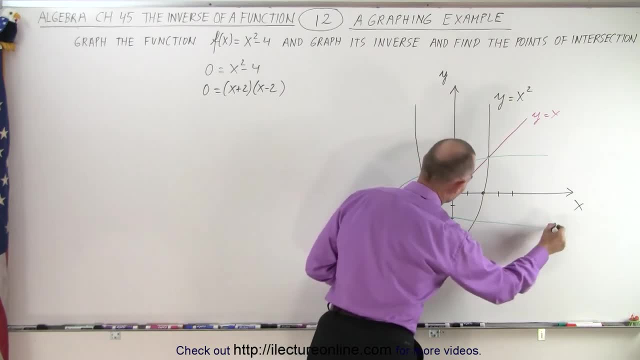 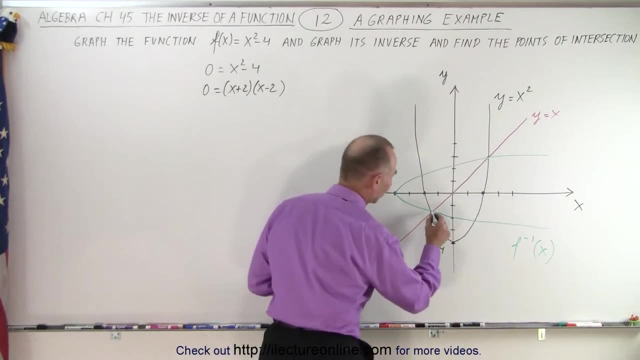 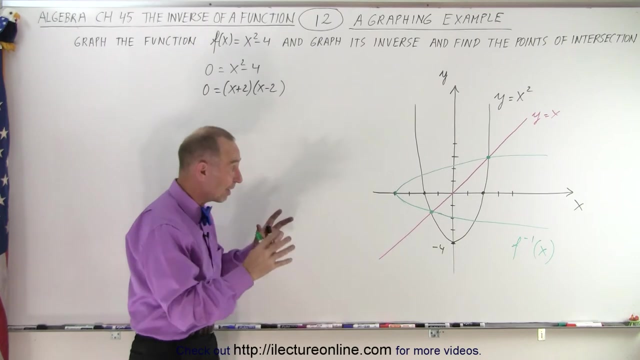 and that point right there and like this. so that would be the inverse of the function. f inverse of the function is the green line. so notice that it crosses the y cos x line at the same place where the function crosses it, and over here as well. so that's how you know that you. 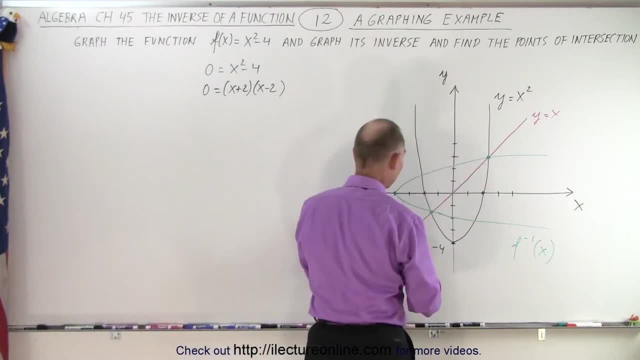 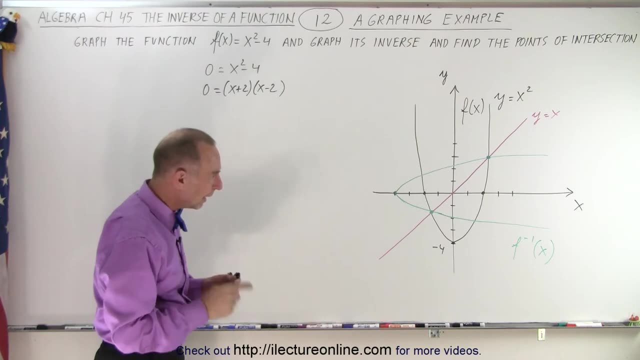 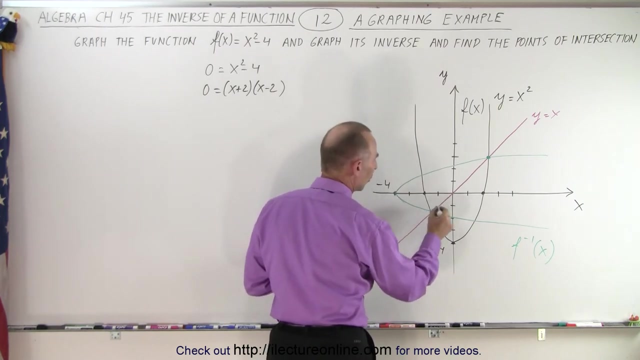 have a graph that is fairly representative. here's the function f of x, so this is f of x. and then here we have, excuse me, the inverse of the function, and you know that the vertice vertex here is at minus four, which means the vertex here is at minus four. so now the question is: what are? 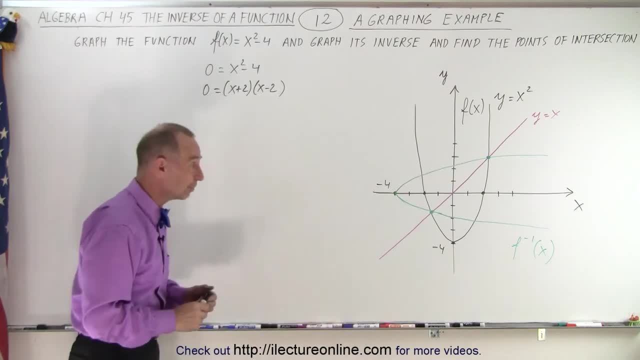 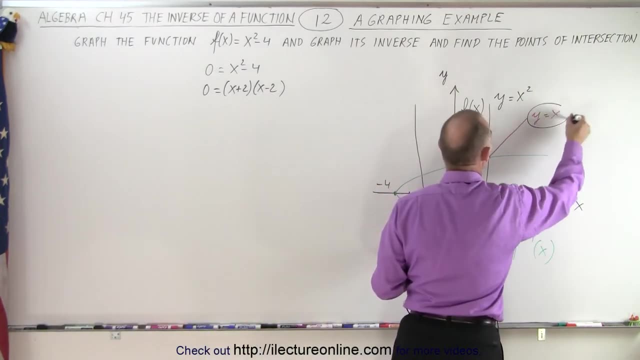 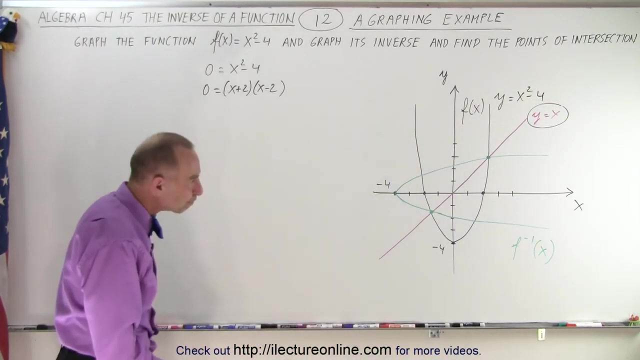 these two points right there, where the two points of intersection between the function and the inverse of the function. We do know that in all cases y equals x. so what we could do? oh, I guess I should be minus four there. that's the function, all right. 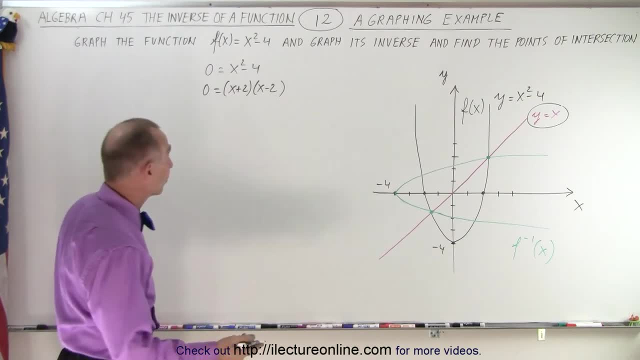 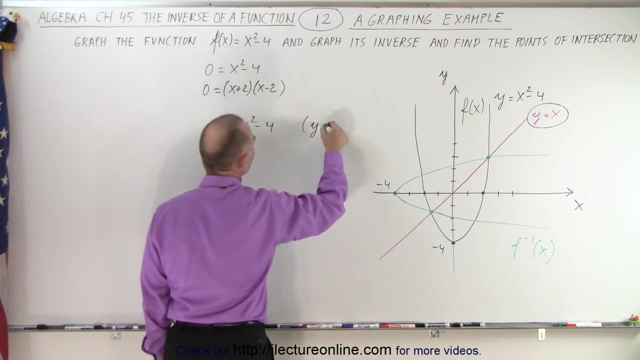 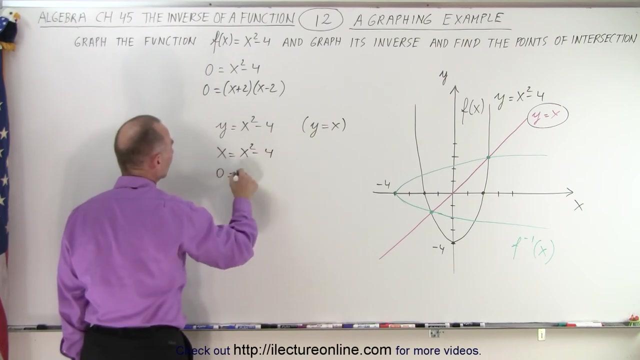 So what we could do is we could set y equal to x. so here we have the function y equals x square minus four, and we know that y equals x, so then I can replace y by x, so we get x equals x square minus four, or zero equals x square minus x minus four. 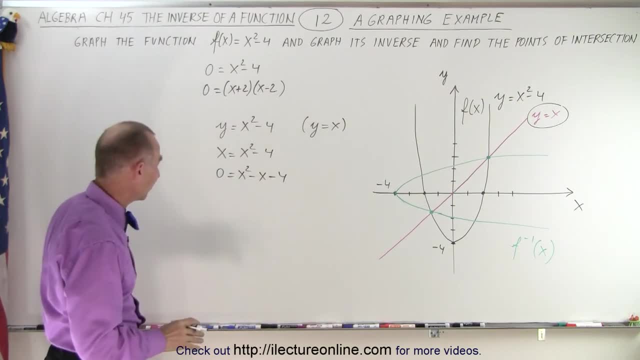 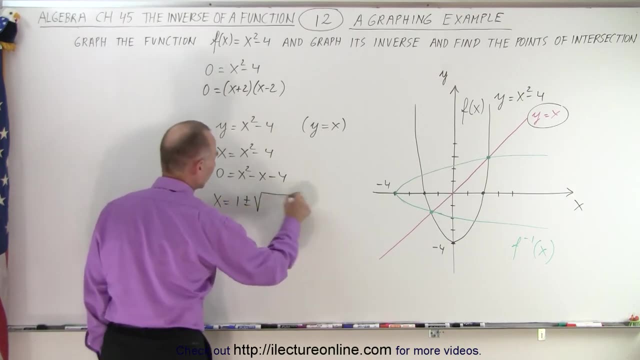 Unfortunately we can't factor that one, so we have to use the quadratic formula that x is equal to minus b, which is one plus or minus the square root of b squared, which is one squared minus four times a times n. 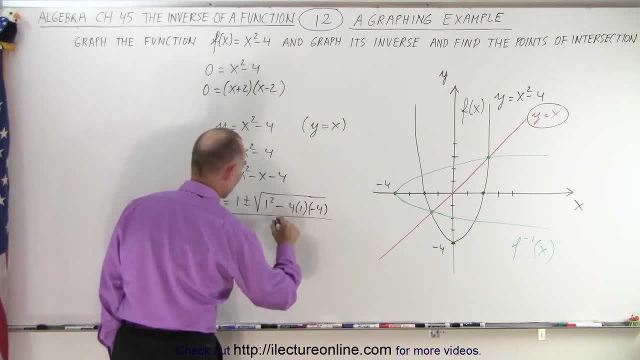 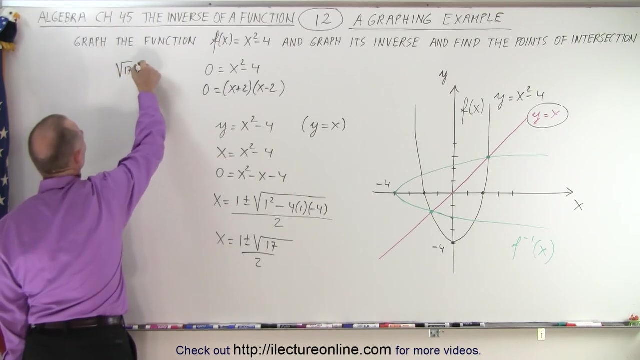 C, which is a minus four, all divided by 2a, which is two. So we get: x is equal to one plus or minus. the square root of that's a positive 16 plus one, that's 17, divided by two, and the square root of 17,. that's about equal to, maybe about. 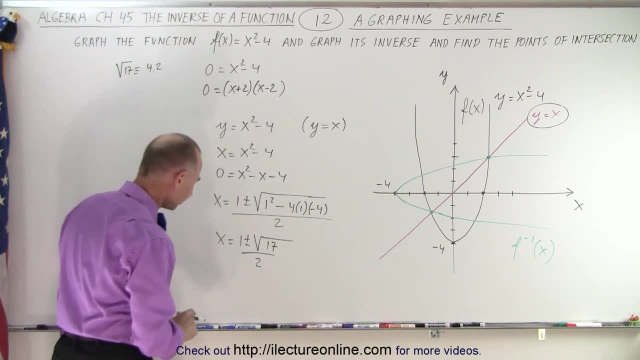 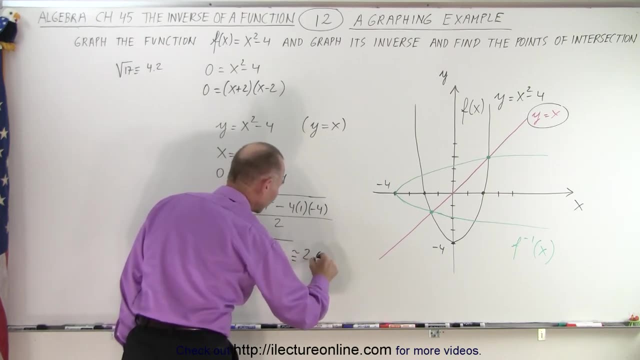 4.2 or something like that close enough. So here that would be equal to 5.2 divided by two. that would be about approximately 2.6.. Or the negative negative 4.2 plus one, that's negative 3.2, divided by two, that would be. 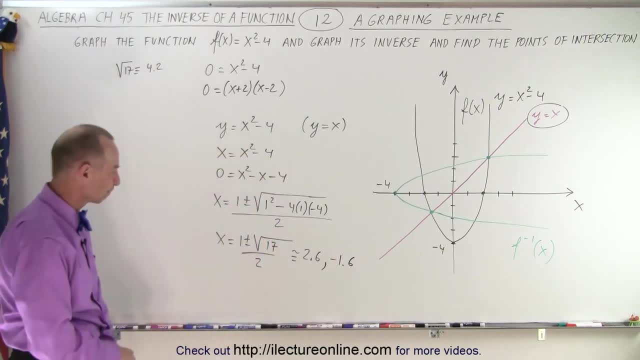 minus 1.6.. There we go, All right. is that about right? 4.2, 5.2 divided by two is 2.6.. 4.2 minus one is 3.2, 1.6.. 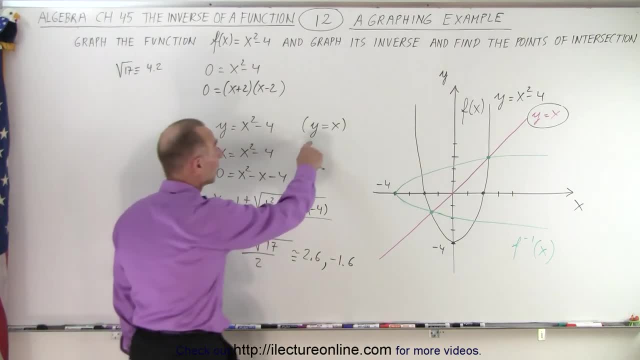 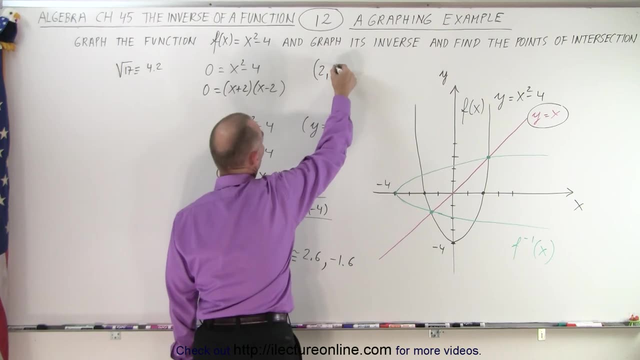 Yep, so those are the two points for x and of course, since y equals x, that also will be the y value. So the two points where they cross that would be at 2.6.. Comma 2.6, that should be a decimal point, right there. 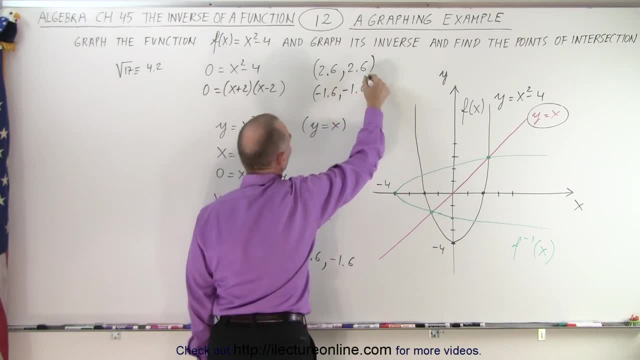 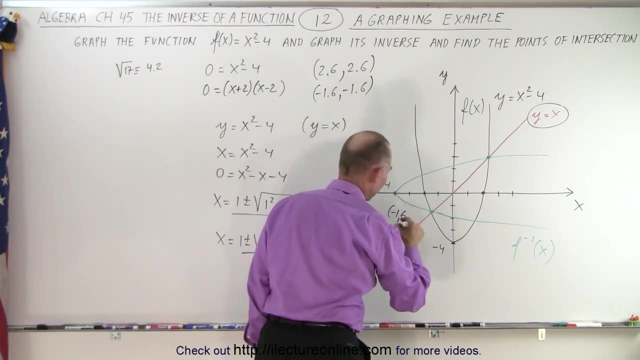 And the other point would be minus 1.6 and minus 1.6.. Can we find those two points Sure enough? there's our first point, right there would be minus 1.6.. I keep putting a comma there. 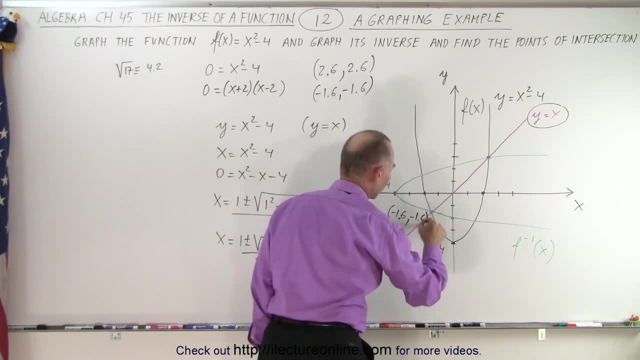 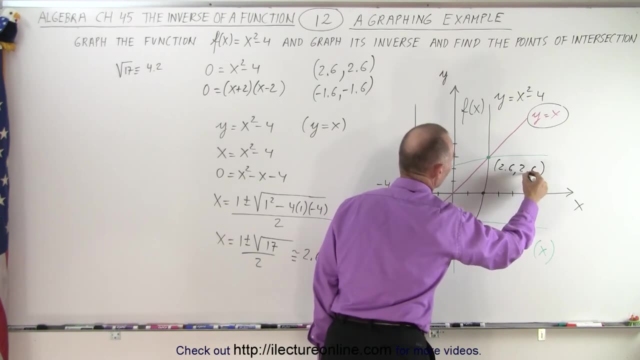 0.6, like that Comma minus 1.6, that's one of them, And over here that would be the point 2.6, comma 2.6.. Oh, that's a decimal point. Too many curves there. 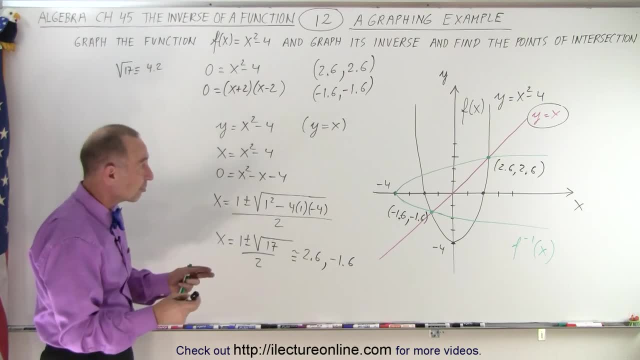 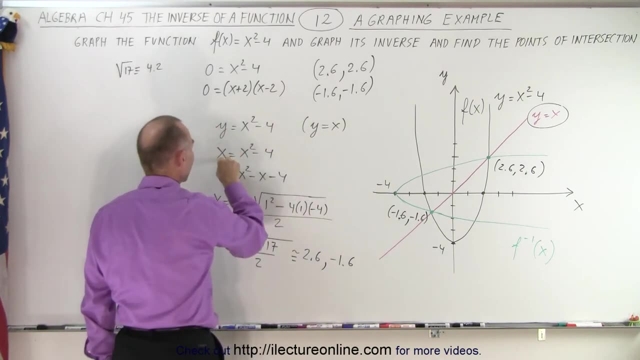 There we go, And that is how we find the two points of intersection between the function and its inverse, realizing that y equals x. So we take the function, we replace y by x, we solve for x and, of course, whatever x. 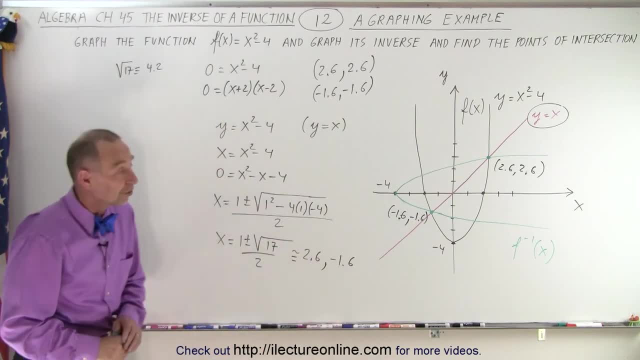 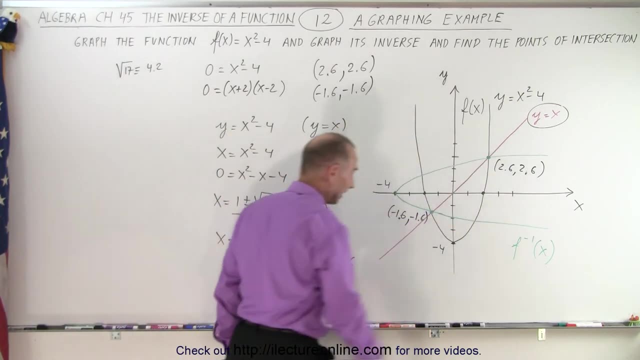 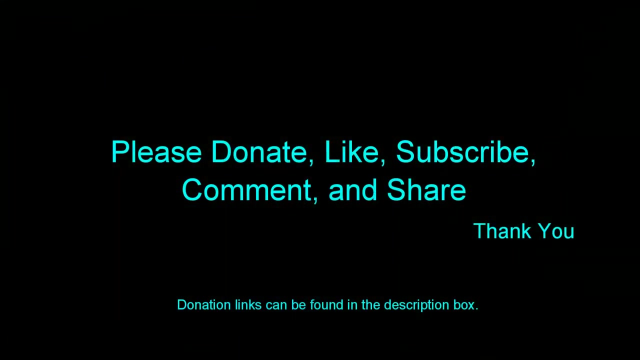 is y is the same thing, And so those are the points of intersection between the function and its inverse, and they always will be on the line y equals x, And that is how it's done. . . . . . .